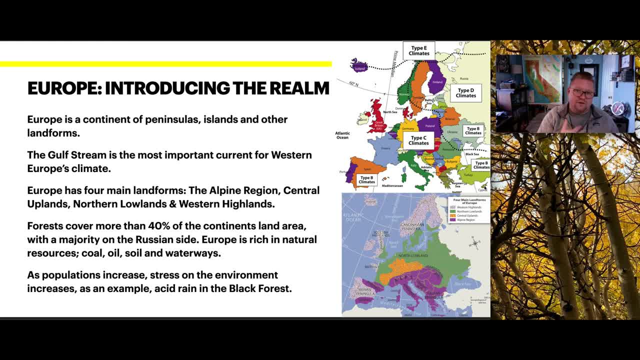 Mediterranean, C being more medium, what more like we have here in Southern California. D is more temperate and then E is a lot colder. So we see there's quite a spectrum of climate And the reason that we have this big change from E to B is because of that Gulf Stream, Now that 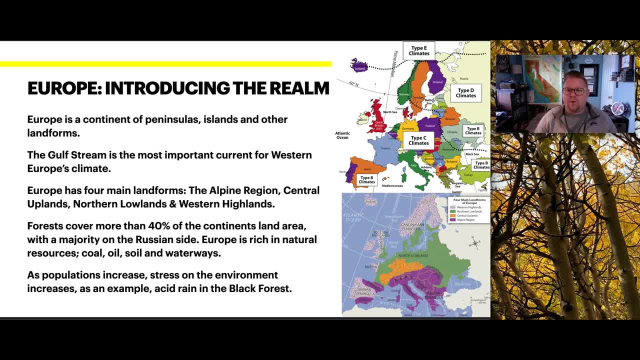 being said, we're going to talk a little bit more about the Gulf Stream. We're going to say we can also divide Europe into four major landforms, which can be observed in the lower right-hand map. We can see we have the Western Highlands. we can see that we have the Northern 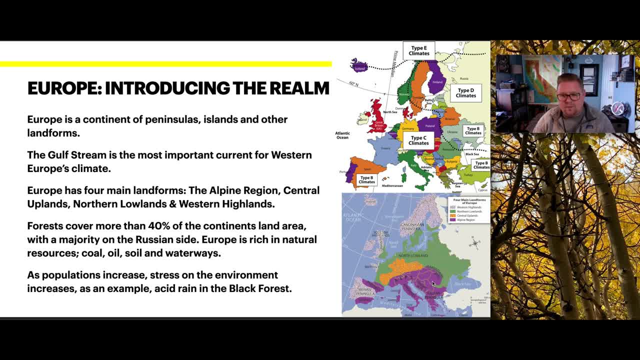 Lowlands, we have the Central Uplands and then the Alpine or Alp region. Now, speaking more on a biological level, Europe itself is as a continent. 40% of the continent is covered in forests. A lot of the continent is covered in forests. So we're going to talk a little bit more about that. 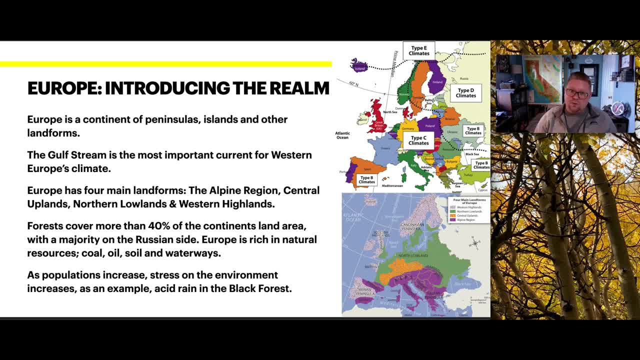 Now, that being said, Europe is still rich in natural resources, Obviously with lumber coal oil, their soil is very fertile- as well as tremendous amounts of radial waterways that allow them to transport and then to provide water for their resources that they're producing Now. 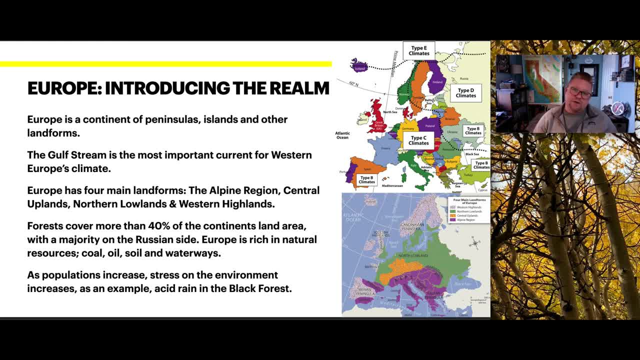 things that have been observed is with population. As populations increase, so does the stress on the environment. The text does a great job using the example of acid rain in the Black Forest, And something to add to the Black Forest is that it's a great example of acid rain in the Black Forest. 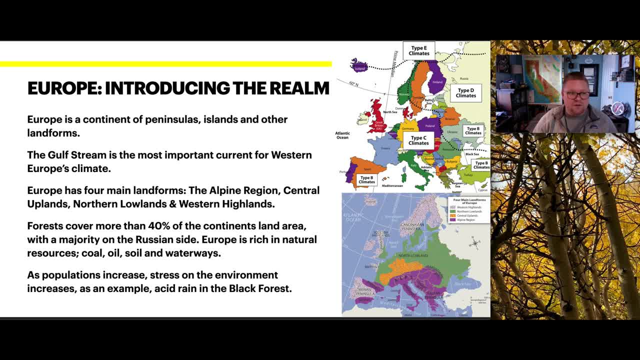 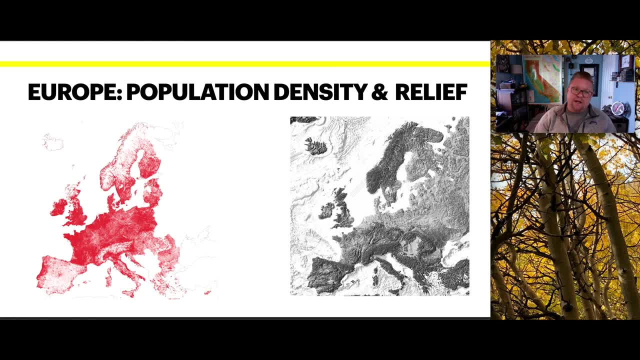 It's not just known for their gummy bears, but they're known for their cuckoo clocks, which required a tremendous amount of lumber. So let's look at a couple other images of Europe. I have on the left, in red, a population density map, meaning that each dot represents a specific volume. 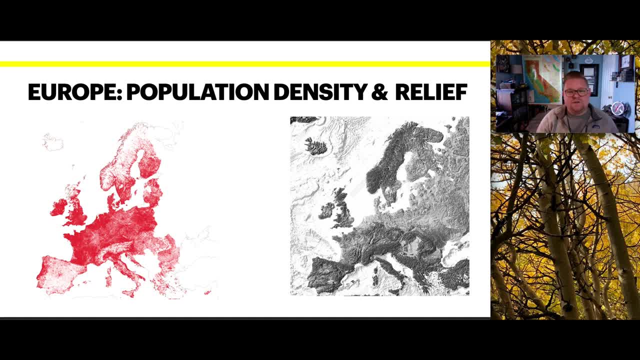 of population. And then on the right hand side is a raised relief using texture to show kind of three dimensions, And we notice that there are some correlations. We see that in areas that are very mountainous, such as this area right here, we see that there are some mountainous areas that 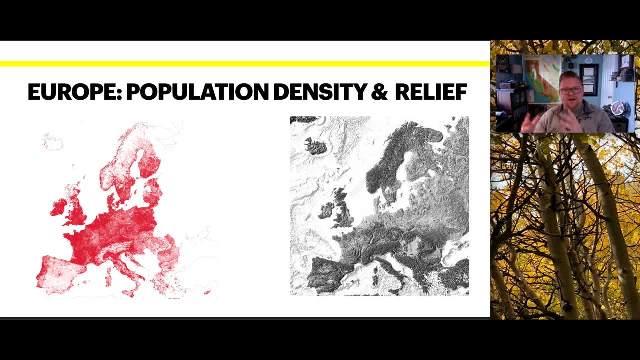 we can see that's observed over here. So we find that there's a correlation with topography as well as where populations reside. We also see there's a correlation where populations want to reside or do not reside, and looking at climates as well, much like we would in California, And so make 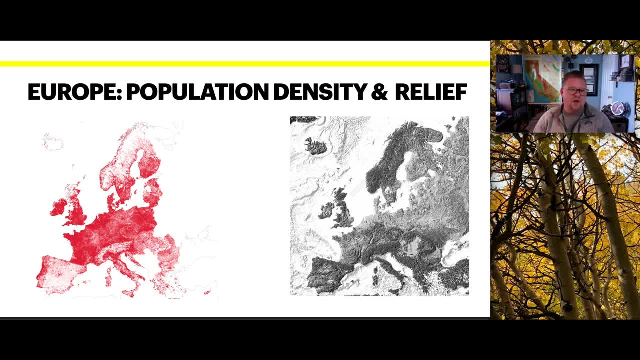 sure you cover some of that material in the text and kind of ask yourself what other patterns are observed. Is there a correlation with where populations live and major waterways for trade and for transport? Moving forward, we can also look at some of the historical development. Now, going back to the 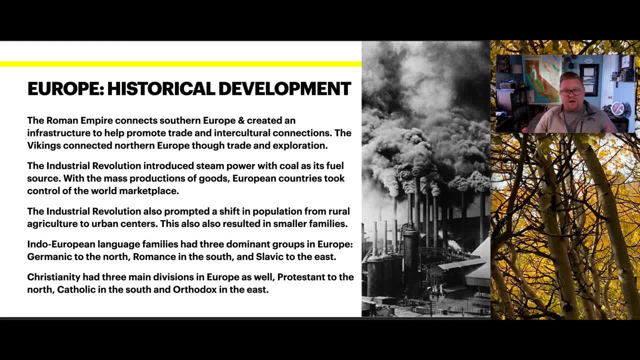 Roman Empire that connected southern Europe and created an infrastructure to help promote trade and intercultural connections across the globe. The Vikings also connected northern Europe through trade and exploration, But it really wasn't until the Industrial Revolution where the invent of steam power, which is powered by coal as a fuel, helped produce a tremendous amount of materials. 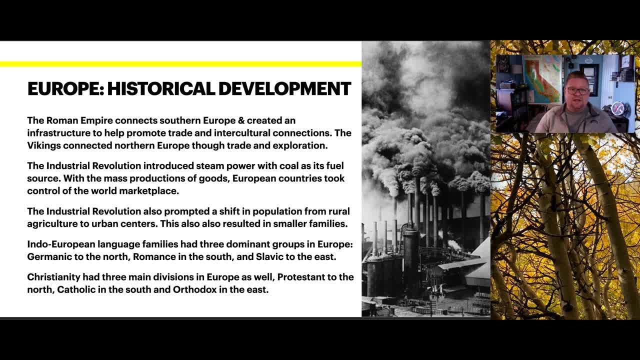 and goods and which really allowed European countries to take advantage of the industrial revolution and take control of the world marketplace. The Industrial Revolution also prompted a shift in population from rural agriculture to urban centers, which also had an effect on population sizes of your family. So, looking at how large families are, Traditionally rural families have larger families. 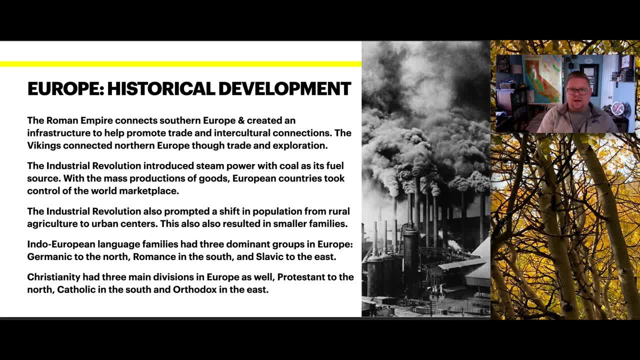 and city families usually have smaller groupings And there's lots of reasons why. an example of that would be: just if you live, if you have your own farm, it's your family farm. it's kind of seen as free labor to have lots of kids to help work for you, And if you have a family farm, it's kind of 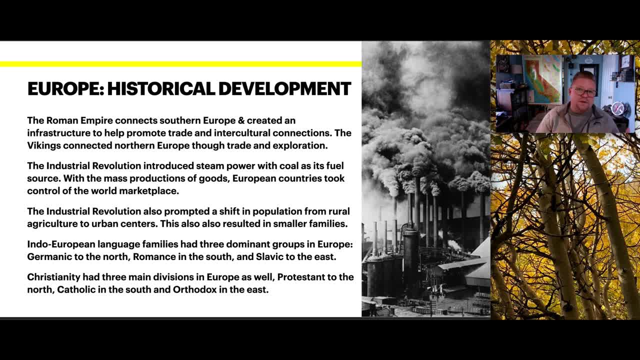 when you're working in a cityscape and having a, you know it's an industrial or business job. you know it's not really a necessity to have so many kids, because you have to be able to support, feed and provide for them. Now, looking at language families, Indo-European language families have 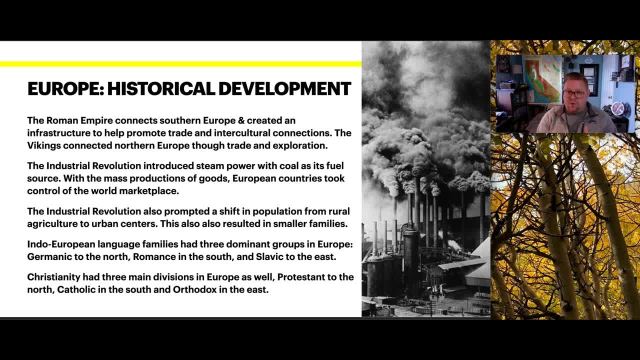 three dominant groups in Europe. You have the Germanic to the north, you have the Romance to South and Slavic to the East, And then, aside from that, looking at religion, we can see that Christianity also has three main divisions. You have Protestant to the north, Catholic to the 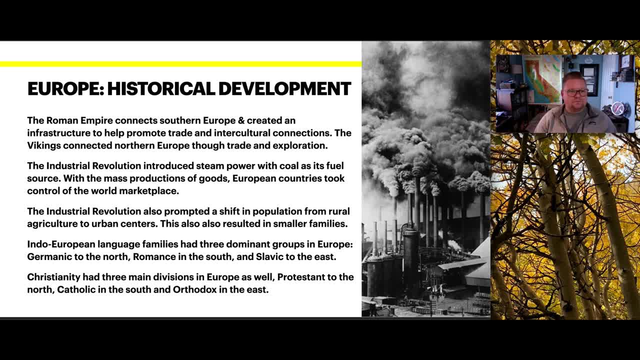 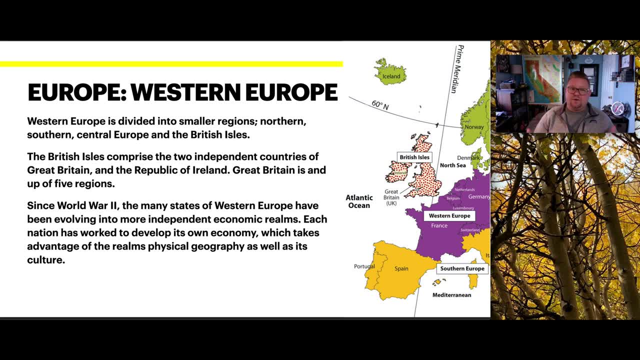 South and Catholic to the West, And then you have the Germanic to the West and then you have the orthodox to the east. now, looking at specifically just western europe, western europe is divided into smaller regions. you have northern, southern, central europe and then the british isles, now the 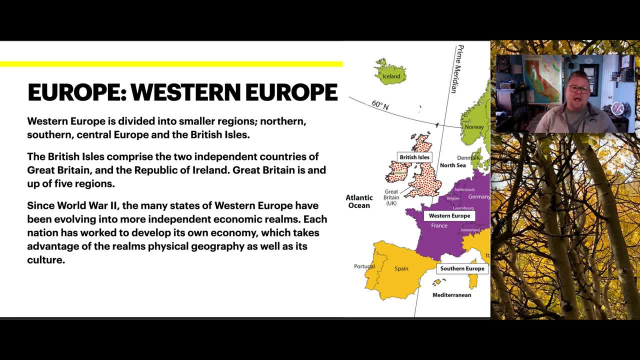 british isles is made up of two independent countries of great britain and the republic of ireland. great britain can also be divided into five smaller regions as well now, since world war ii, many of the states in western europe have been evolving into more independent economies. 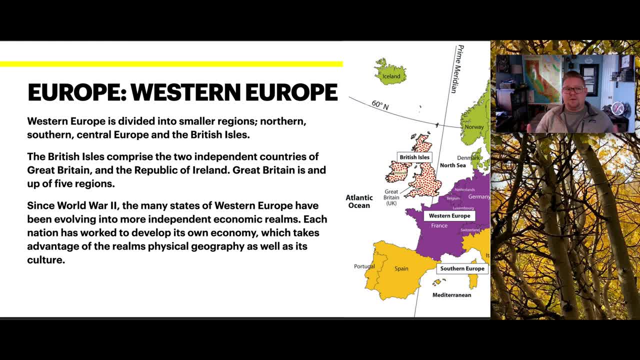 and realms. each nation has worked to develop its own economy which takes advantage of the realm's physical geography resources as well as the culture. now the eastern europe has a little bit of a different story. so after world war ii europe was divided from west to east by the iron. 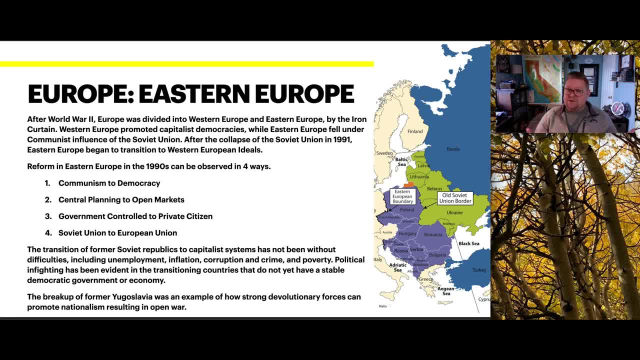 curtain. western europe promoted capitalist democracies, while eastern europe fell under communist influence of the soviet union. now, after the collapse of the soviet union in 1991, eastern europe slowly began transitioning to western european ideals. so reform in eastern europe in the 1990s can be absorbed. it was 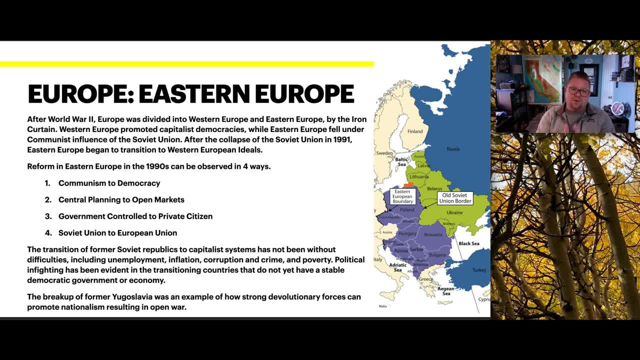 observed, excuse me, in four ways. one was that it went from communism to democracy. the second was that central planning went to a open market government, controlled, moved to private citizen, and then, lastly, the soviet union and then merging into then the european union. the transition of 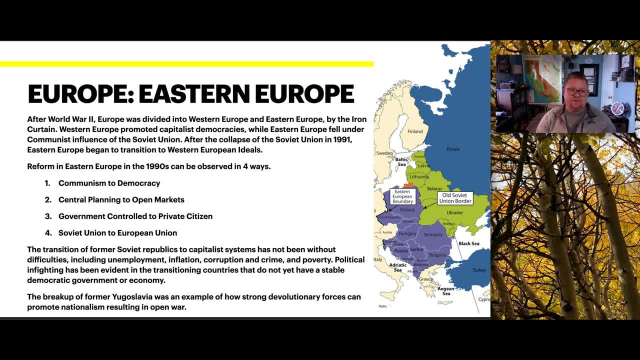 former soviet republics to capitalist systems have not been without difficulty, and that's why we have a lot of difficulties, including unemployment, inflation, corruption, crime and poverty. political infighting has been evident in the transition as well. the breakup of former yugoslavia is a great example of how strong 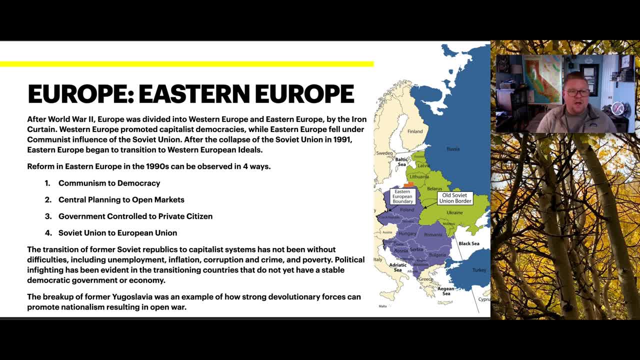 devolutionary forces can promote. nationalism results in open war. so when the iron curtain went down, which many of us know is the berlin wall- and i actually have a piece of the berlin wall that i wanted to share with you, so this was a friend of mine who lives in germany- when he moved. 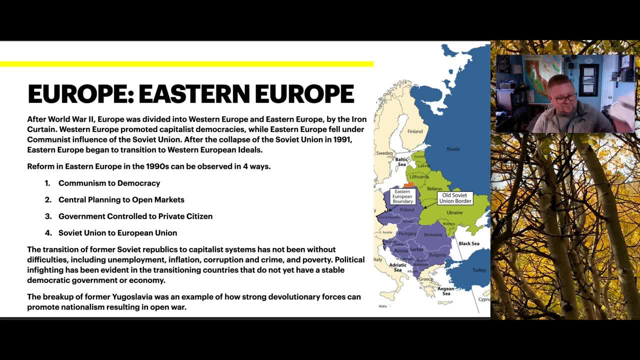 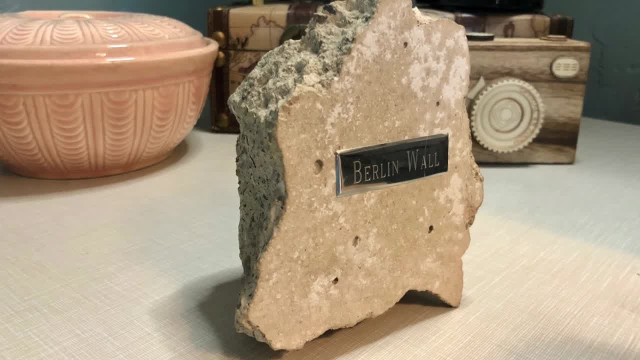 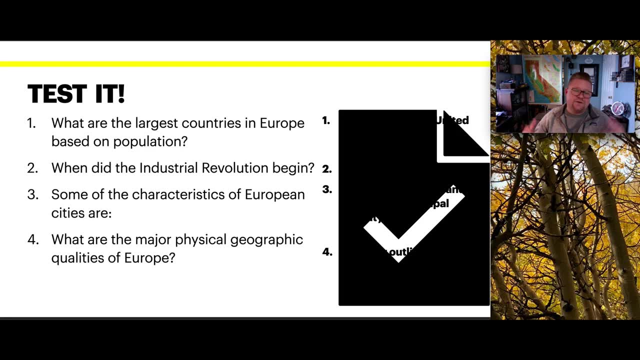 to germany and he brought a couple pieces for a few of us of the pieces of the berlin wall. so let's test your european knowledge. here's some four questions that come from the reading as well as from the video, and see if you can plug in your own answers. the first one is: what are the 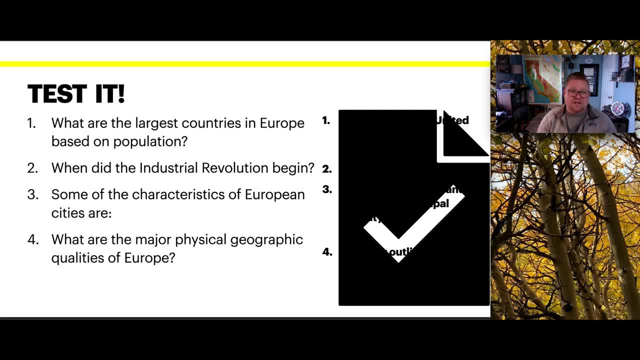 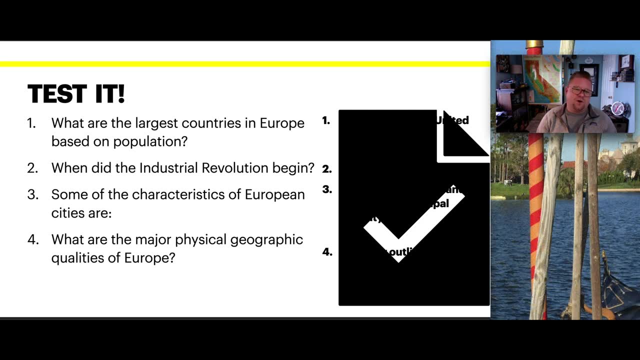 largest countries in europe based on population? and the second one is: when did the industrial revolution begin? the third question are some of the character characteristics of european cities can be or are? and the final question are: what are the major physical geographic qualities of europe? so i'm going to leave those questions there for a moment. things you should, you know, really walk.